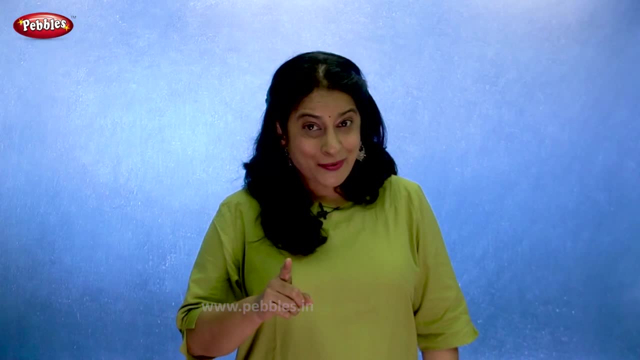 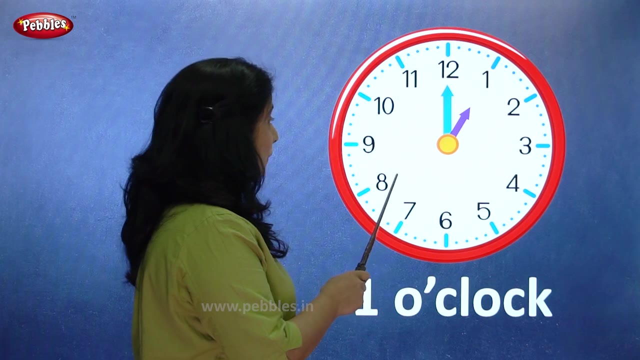 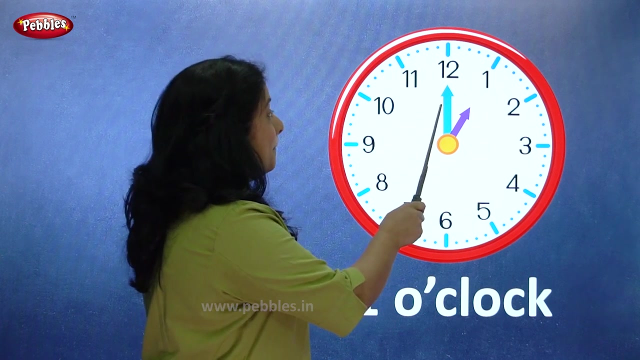 Hello friends, how are you? Today we are going to learn about the clock and the time, So let's start. This is a clock. A clock tells us time. A clock has two hands: Big hand, small hand. Big hand is called as minute hand, Small hand is called as hour hand. 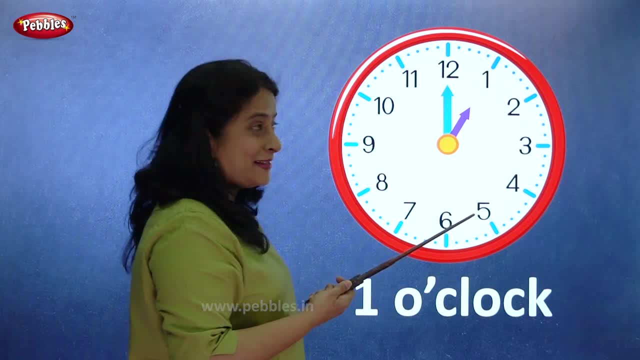 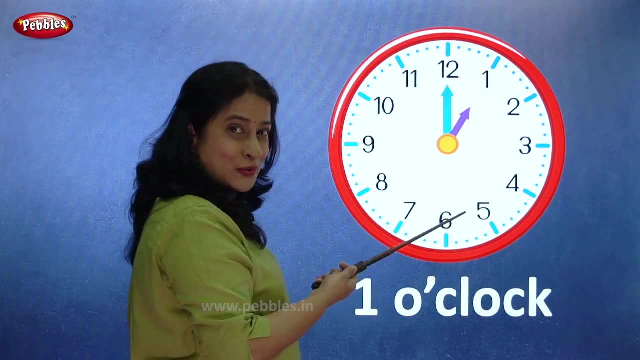 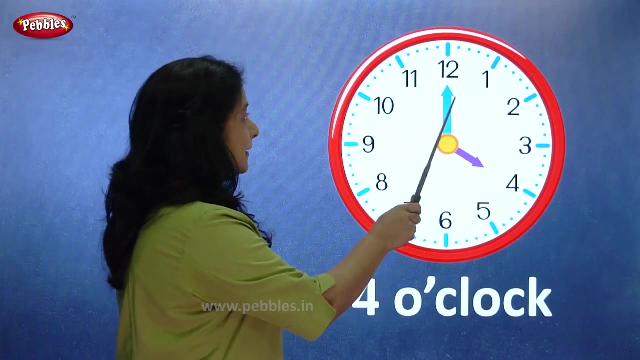 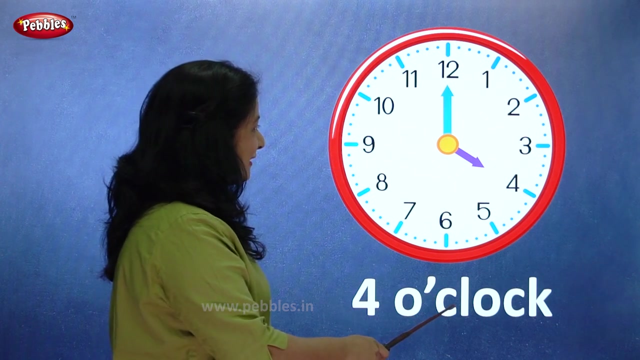 In this example the clock tells us the minute hand is on 12.. The hour hand is on 1. So the time is 1 o'clock. Hour hand is on 4.. Minute hand is on 12. So the time is 4 o'clock. 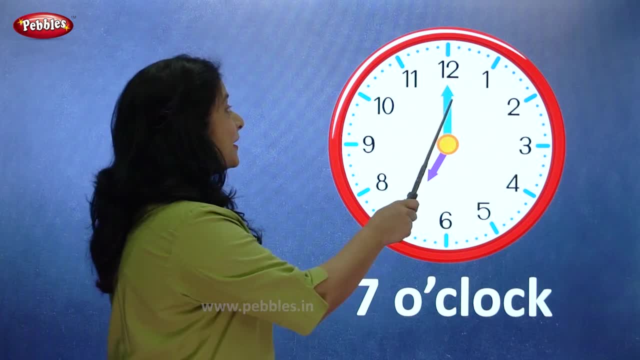 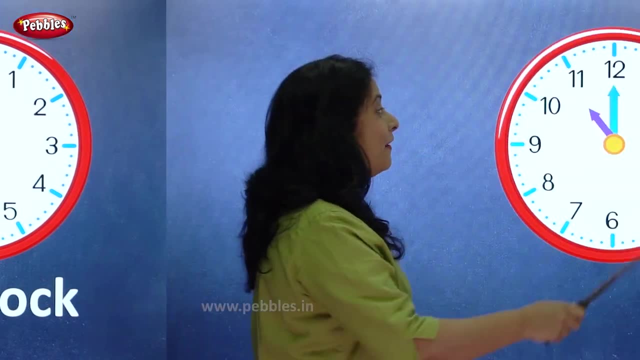 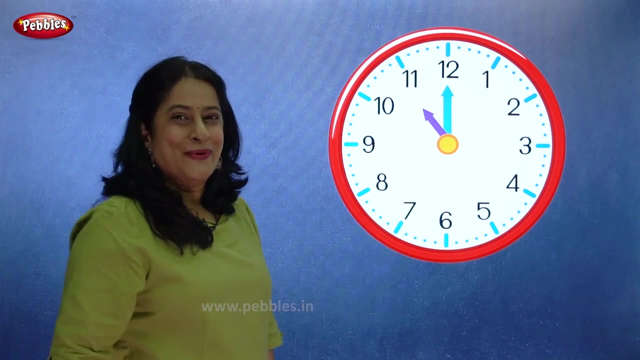 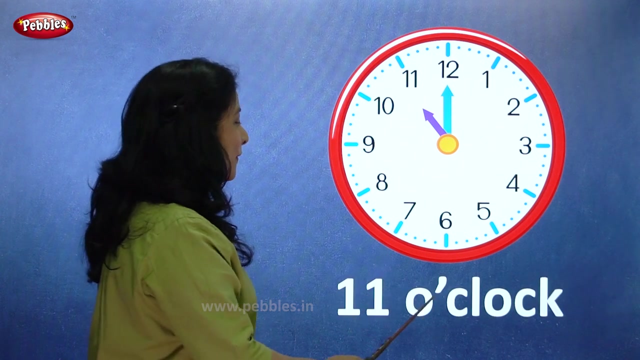 Hour hand is on 7.. Minute hand is on 12.. So the time is 7 o'clock. The hour hand is on 11.. The minute hand is on 12.. So what is the time? Come on, tell me fast. Correct 11 o'clock. 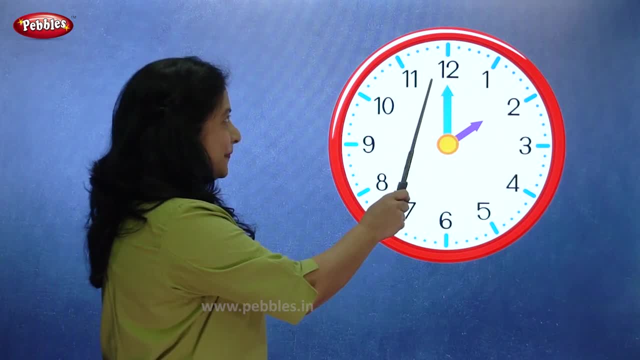 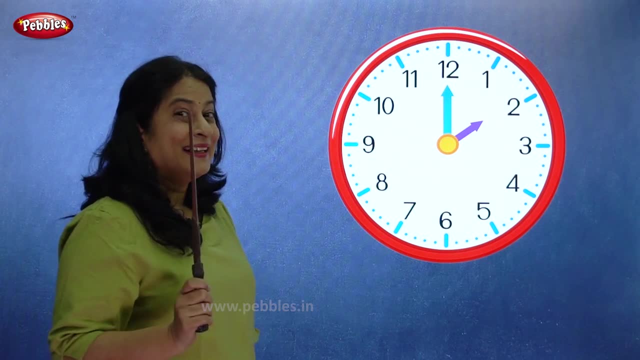 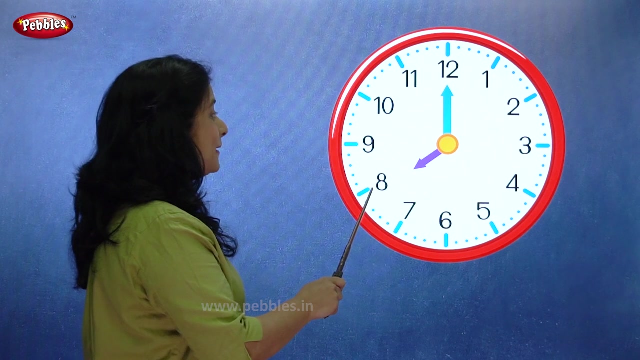 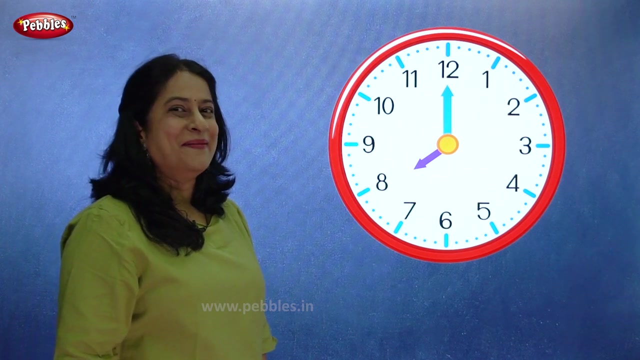 The hour hand is on 2.. The minute hand is on 12.. So what is the time? Come on, tell me Correct, 2 o'clock. The hour hand is on 8.. The minute hand is on 12.. So what is the time? Come on, tell me fast, Correct 8 o'clock. 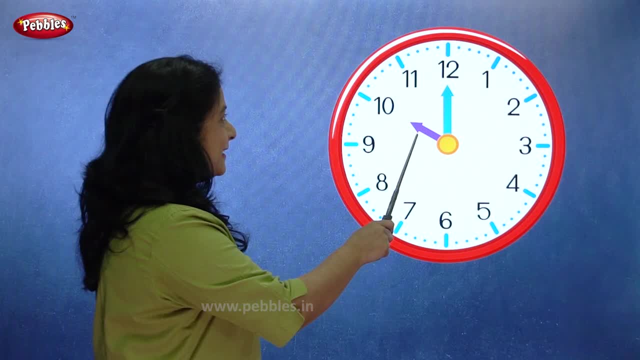 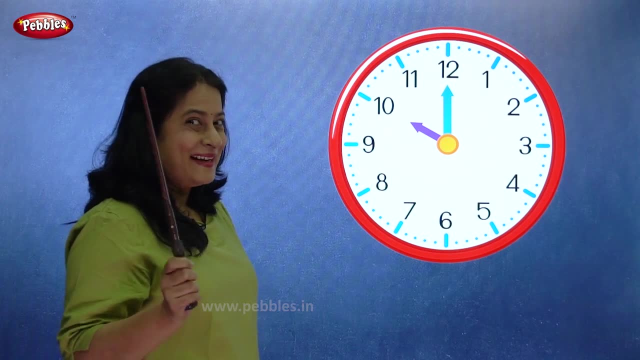 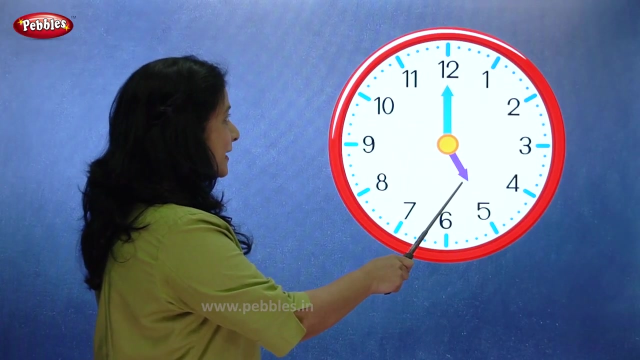 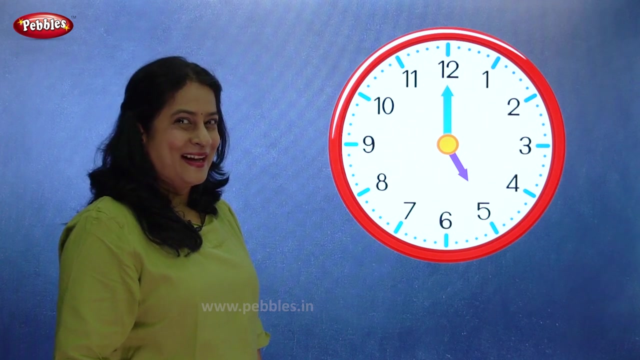 The hour hand is on 10.. The minute hand is on 12.. So what is the time? Correct 10 o'clock. The hour hand is on 5.. The minute hand is on 12.. So what is the time? Come on, tell me fast. Correct 5 o'clock. 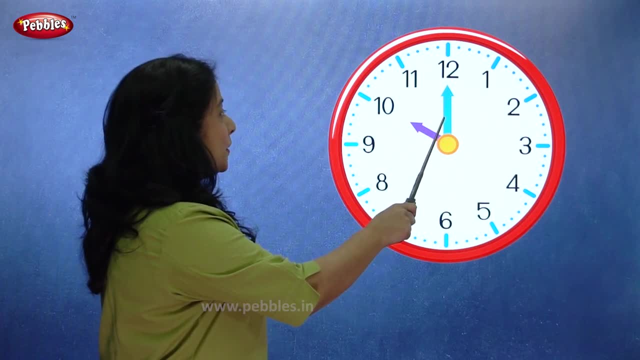 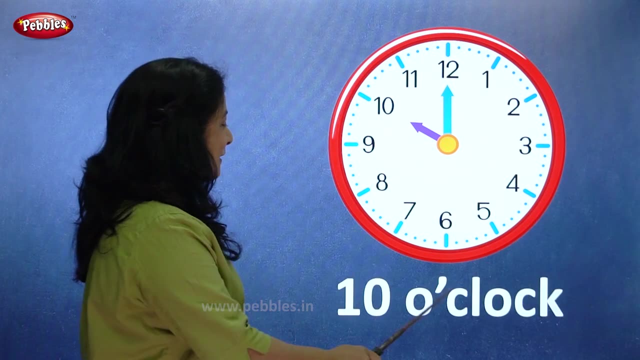 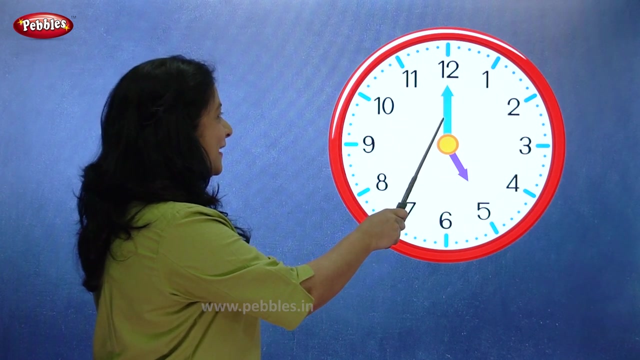 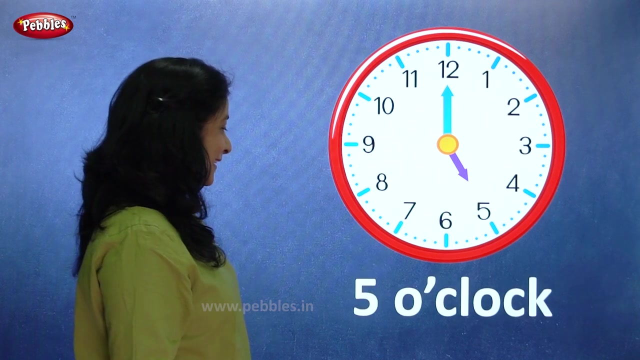 10. the minute hand is on 12. so what is the time? correct? 10 o'clock. the hour hand is on 5. the minute hand is on 12. so what is the time? come on, tell me fast, correct 5 o'clock. the hour hand is on. 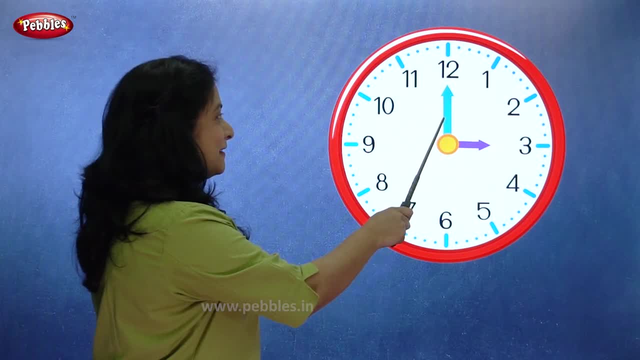 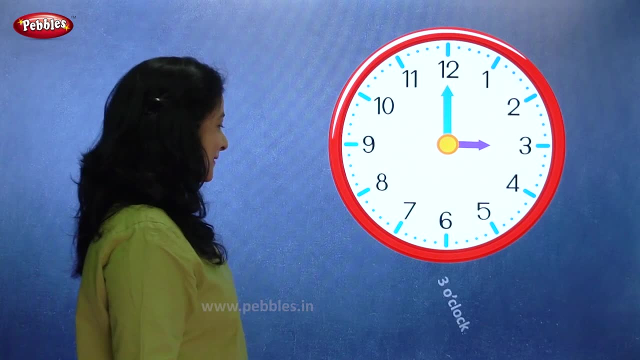 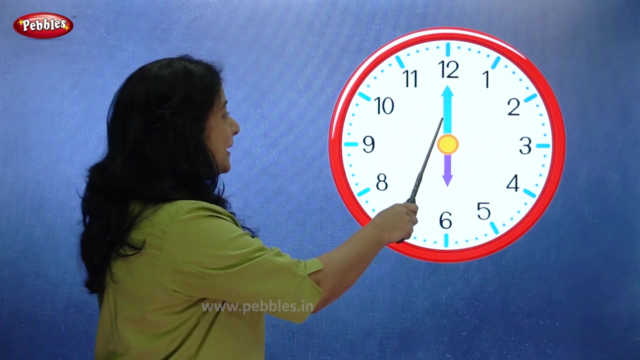 12. so what is the time? come on, tell me fast, correct 5 o'clock. the hour hand is on 3, the minute hand is on 12. so what is the time? come on, tell me fast, correct 3 o'clock. the hour hand is on 6, the minute hand is on 12. so what is the time come? 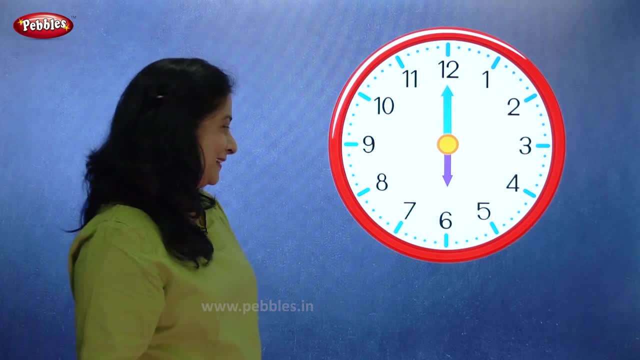 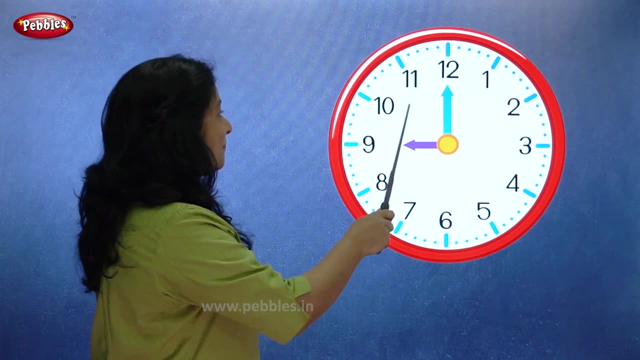 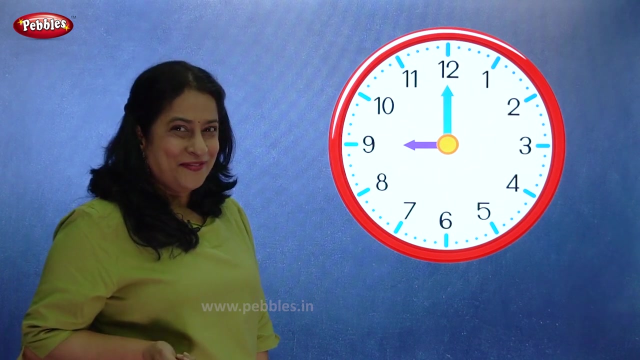 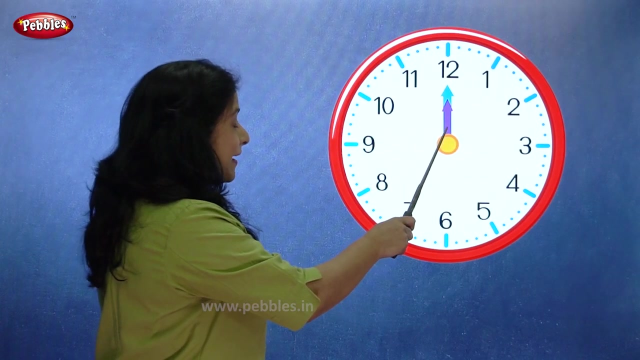 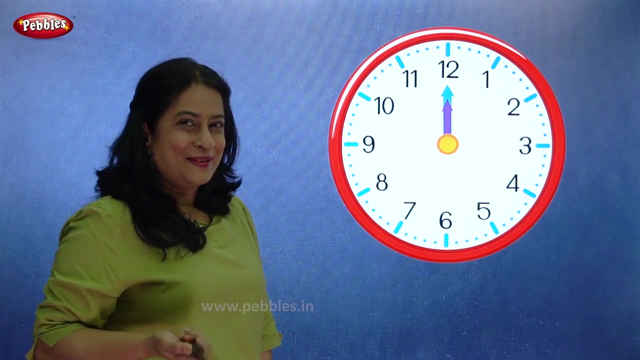 on who's going to tell me? correct 6 o'clock. the hour hand is on 9. the minute hand is on 12. so what is the time? come on, tell me fast. correct 9 o'clock. the hour hand is on 12. the minute hand is also on 12. so come on now tell me the. 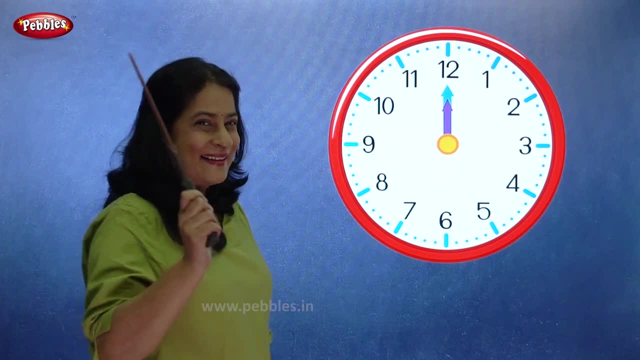 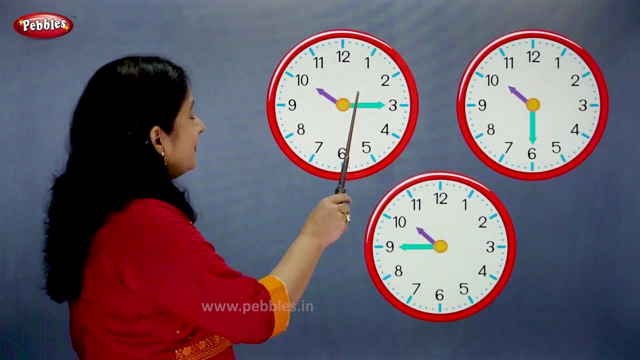 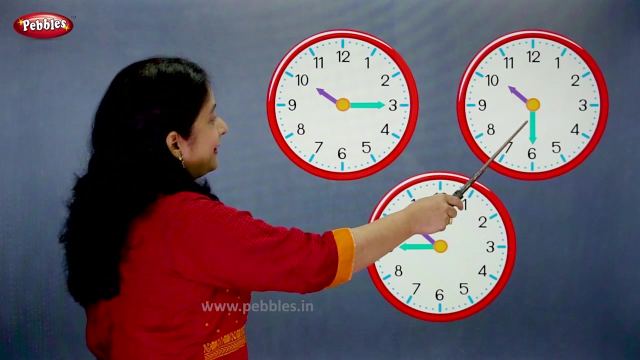 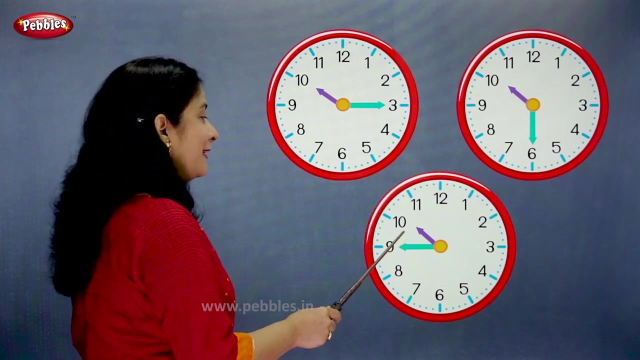 time. tell me fast, correct 12 o'clock. when the minute hand is on 3, we say quarter past the current hour. when the minute hand is on 6, we say half past the past the current hour. When the minute hand is on 9, we say quarter to the next hour. 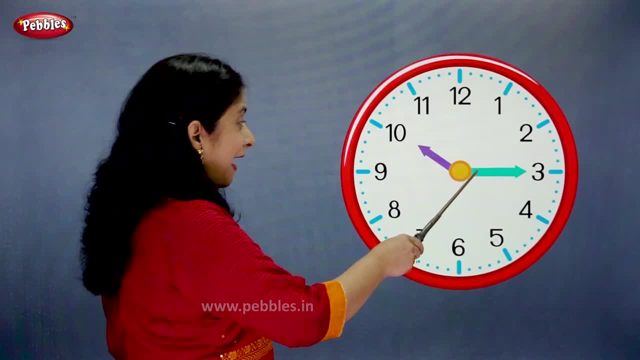 Now let's see some examples. The minute hand is on 3.. The hour hand is on 10.. So we say the time is quarter past 10.. The minute hand is on 3.. The hour hand is on 8.. So we say: 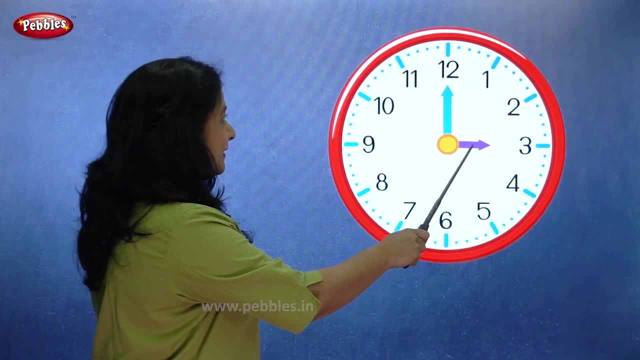 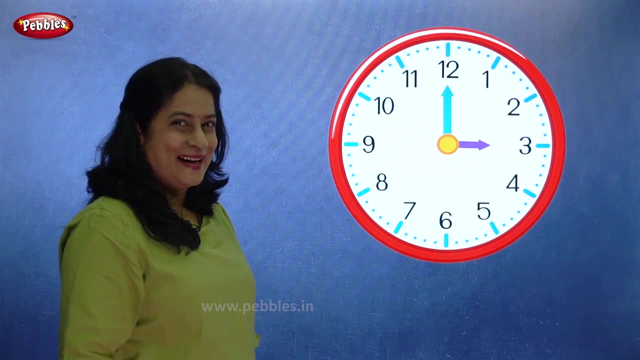 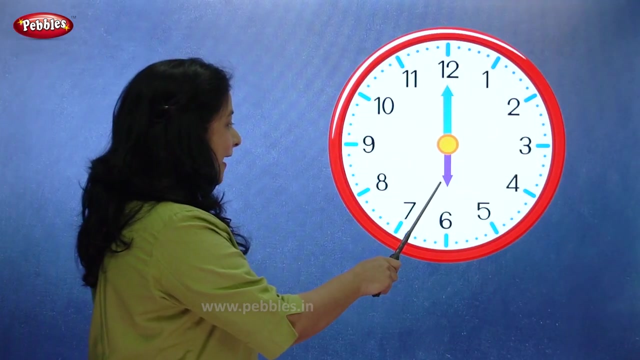 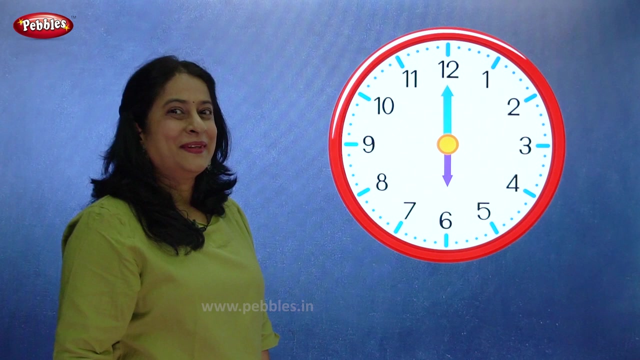 The hour hand is on 3.. The minute hand is on 12.. So what is the time? Come on, tell me fast, Correct 3 o'clock. The hour hand is on 6.. The minute hand is on 12.. So what is the time? Come on, who's going to tell me Correct? 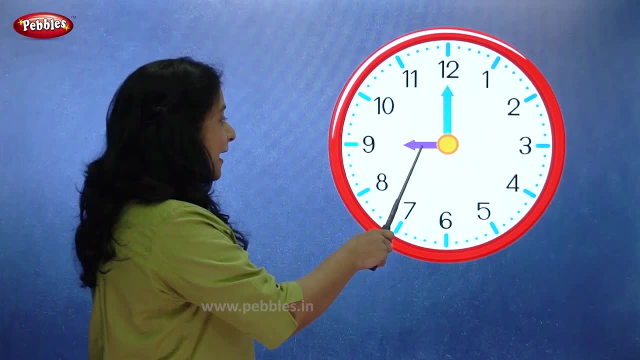 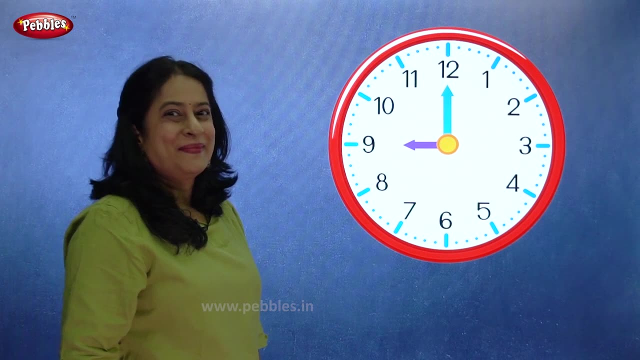 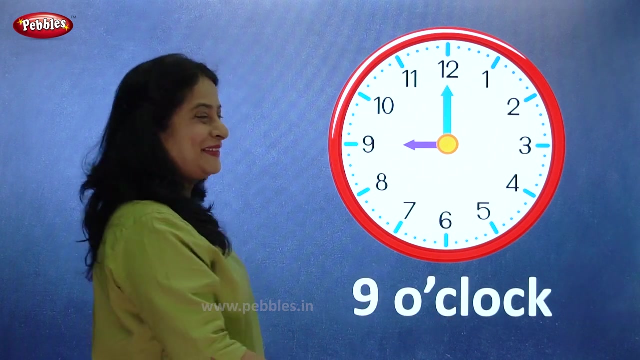 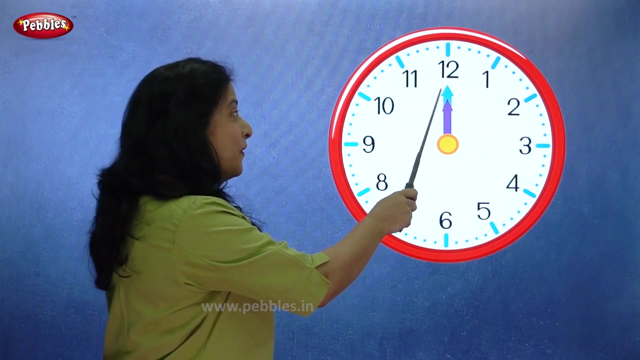 6 o'clock. The hour hand is on 9.. The minute hand is on 12.. So what is the time? Come on, tell me fast. Correct 9 o'clock. The hour hand is on 12.. The minute hand is also on 12.. So come on now tell me the time. 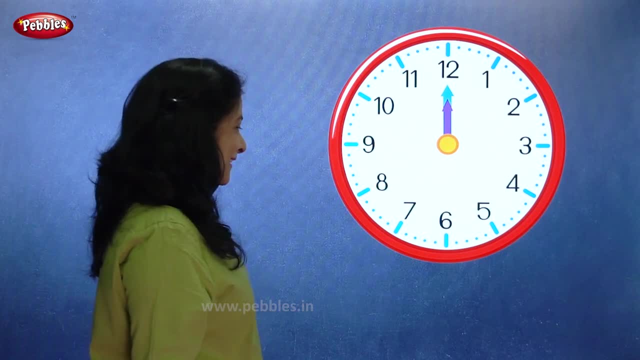 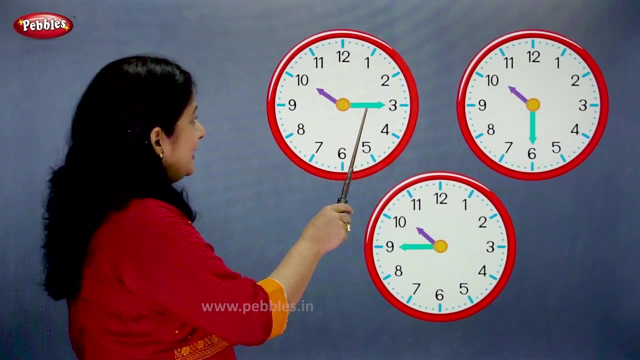 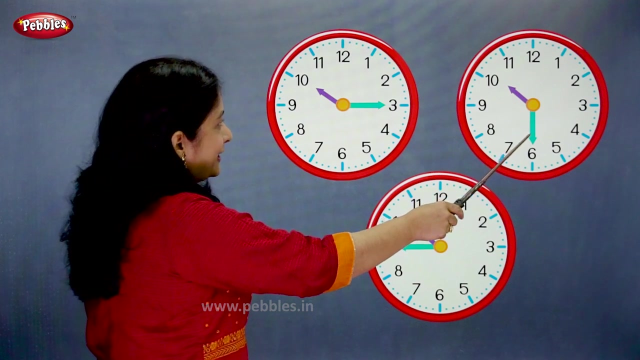 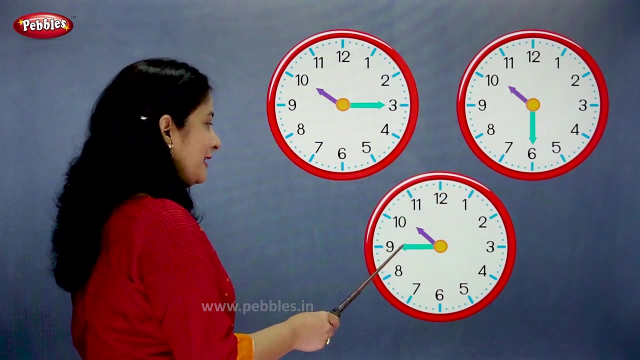 Tell me fast, Correct 12 o'clock. When the minute hand is on 3,, we say quarter past the current hour. When the minute hand is on 6, we say half past the current hour. When the minute hand is on 9,, we say quarter to the next hour. 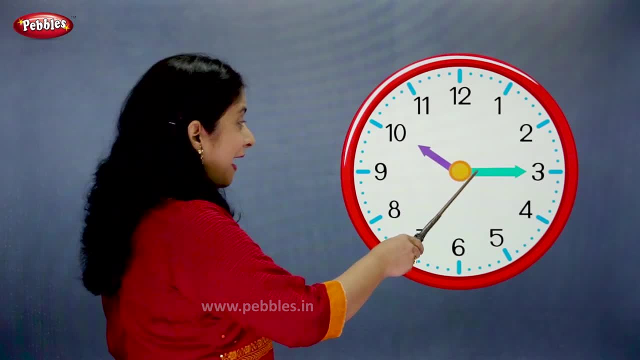 Now, let's see the time, Let's see the time. Let's see the time. Let's see some examples. The minute hand is on 3.. The hour hand is on 10.. So we say the time is quarter past 10.. 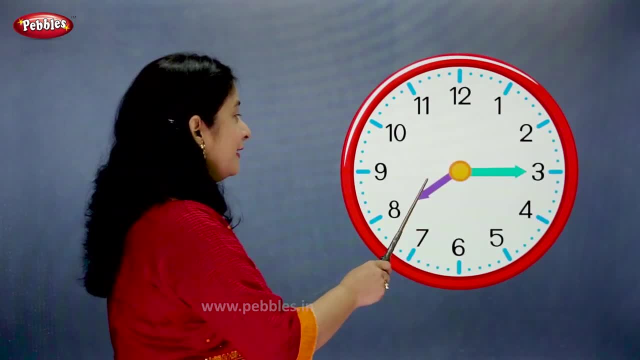 The minute hand is on 3.. The hour hand is on 8.. So we say the time is quarter past 8.. The minute hand is on 3.. The hour hand is on 5.. So we say the time is quarter past 5.. 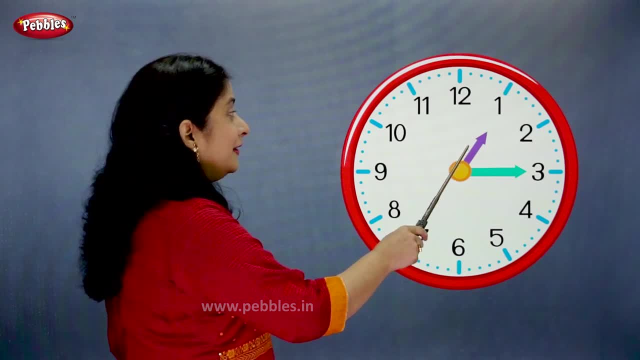 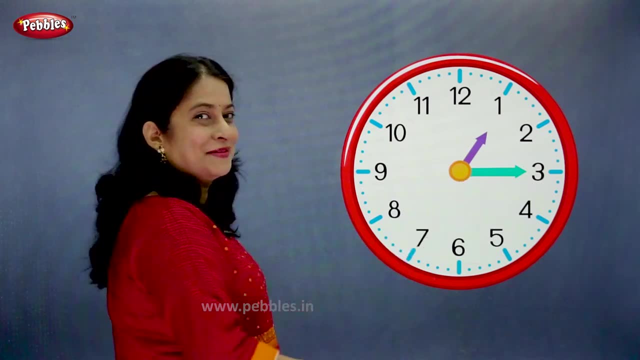 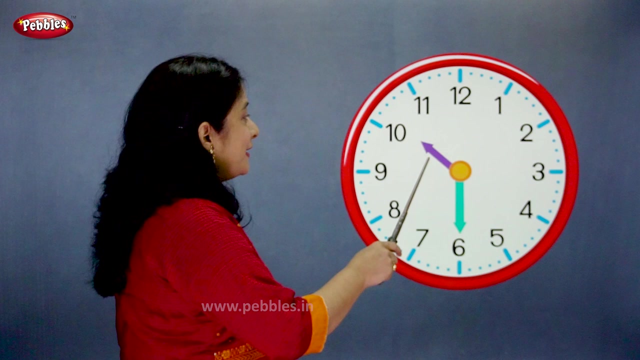 The minute hand is on 3.. The hour hand is on 1.. So we say the time is quarter past 1.. The minute hand is on 6.. The hour hand has passed 10.. So we say the time is half past 10.. 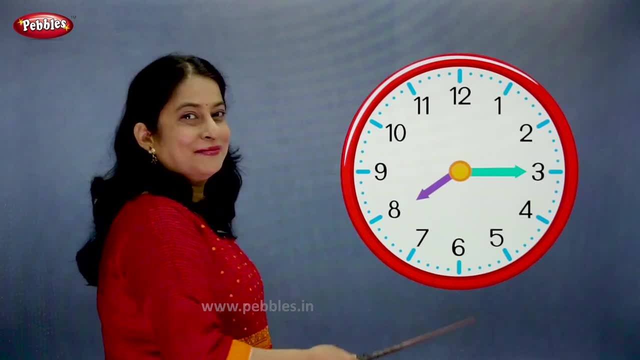 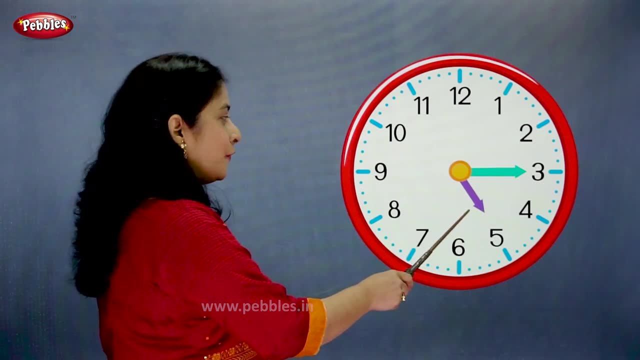 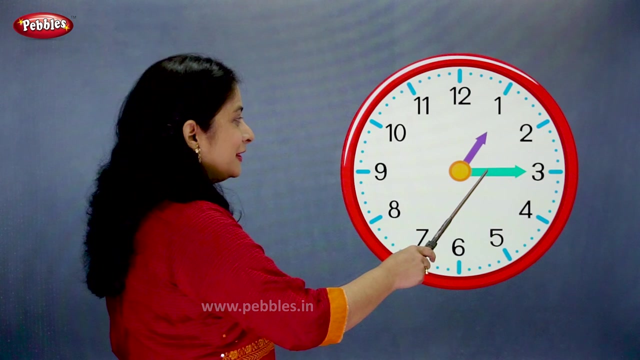 the time is quarter past 8.. The minute hand is on 3.. The hour hand is on 5.. So we say the time is quarter past 5.. The minute hand is on 3.. The hour hand is on 1.. So we say the time is quarter past 1.. The minute hand is on 6.. 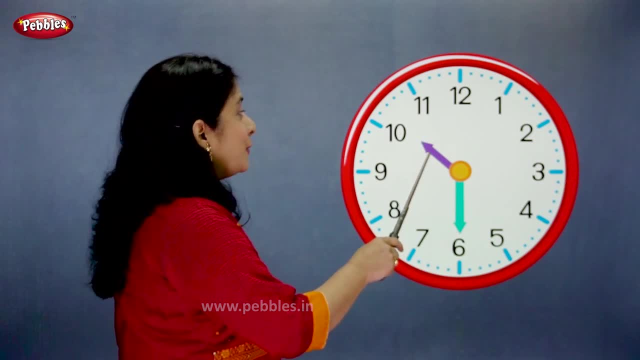 The hour hand has passed 10.. So we say the time is half past 10.. The minute hand is on 6.. The hour hand has passed 2.. So we say the time is half past 2.. The minute hand is on 6.. The hour hand has passed 9.. So we say the time is half past 9.. The minute hand is on 6.. 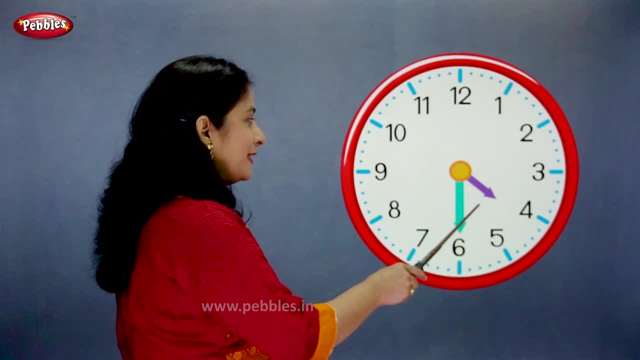 The hour hand has passed 4.. So we say the time is half past 4.. The minute hand is on 9.. The hour hand is moving towards 11.. So we say the time is quarter to 11.. The minute hand is on 9. The hour. 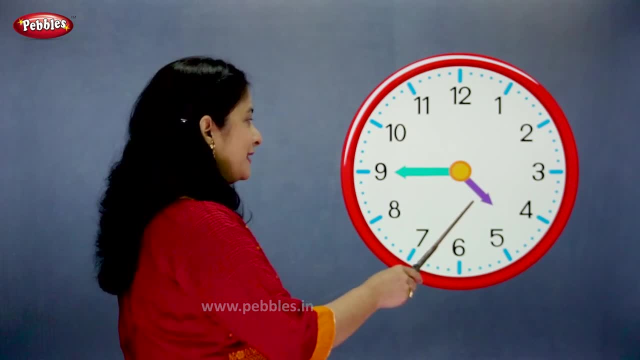 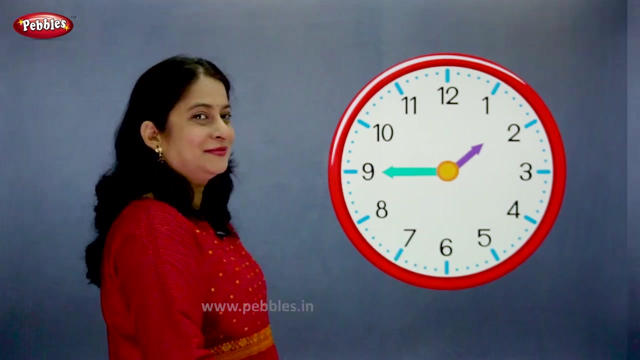 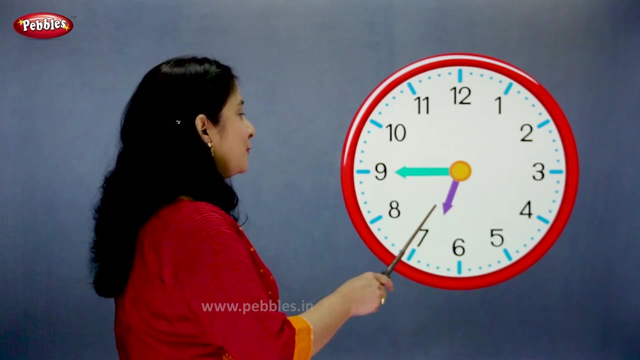 hand is moving towards 5.. So we say the time is quarter to 5.. The minute hand is on 9.. The hour hand is moving towards 2.. So we say the time is quarter to 2.. The minute hand is on 9.. The hour hand is moving towards 7.. So we say the time is quarter to 7.. 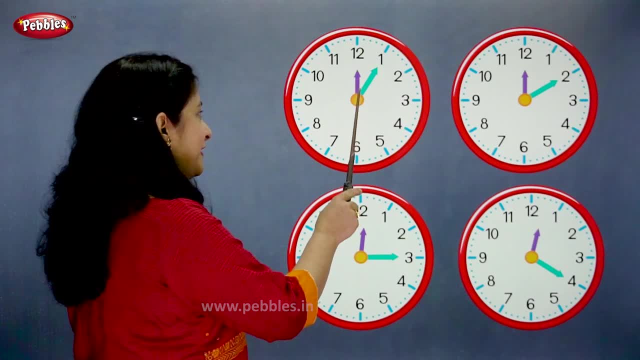 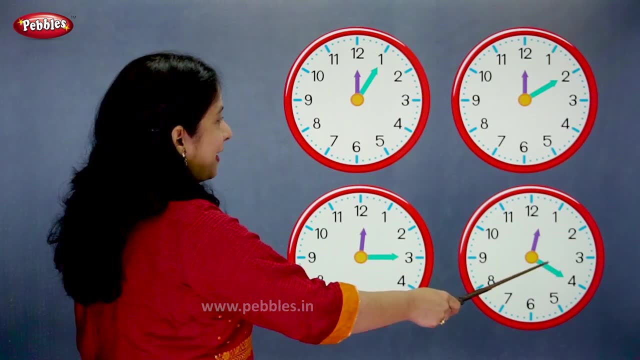 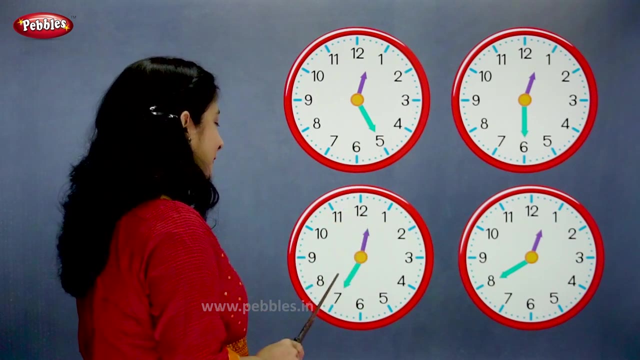 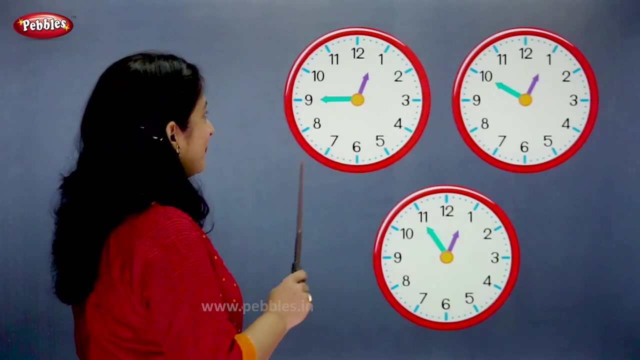 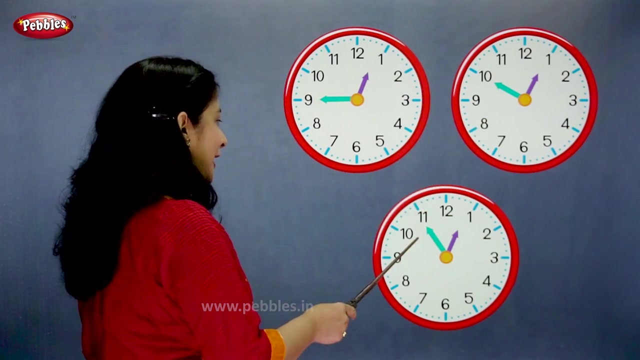 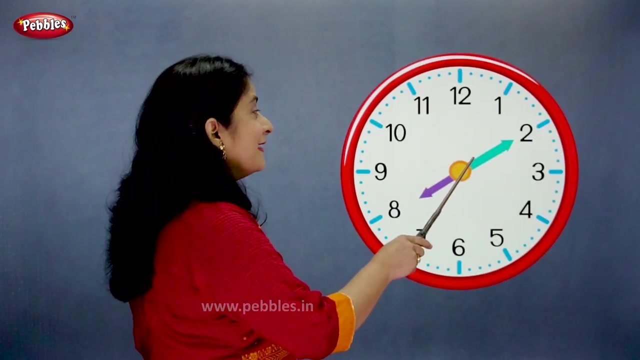 When the minute hand is on 1, we say: 5 passed 10, passed quarter, passed 20, passed 25, passed half, passed 25, 2. 20, 2. Quarter 2. 10,, 2. 5, 2.. Now let's see some examples. The minute hand is on 2. The hour. 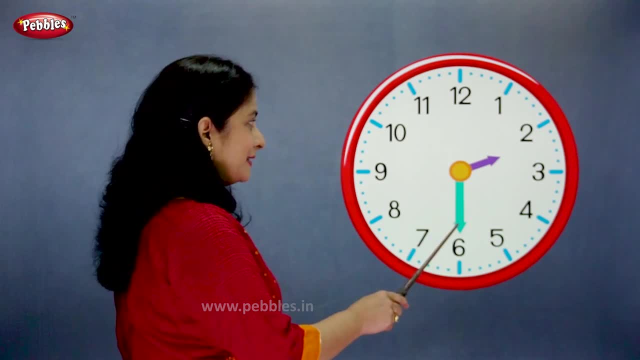 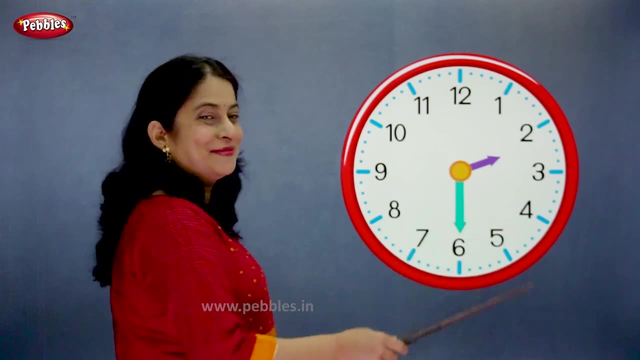 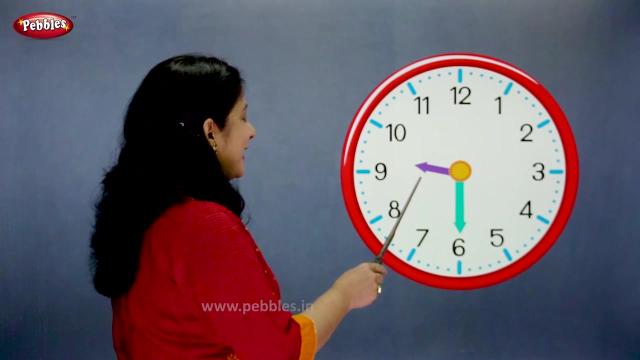 The minute hand is on 6.. The hour hand has passed 2.. So we say the time is half past 2.. The minute hand is on 6.. The hour hand has passed 9.. So we say the time is half past 9.. 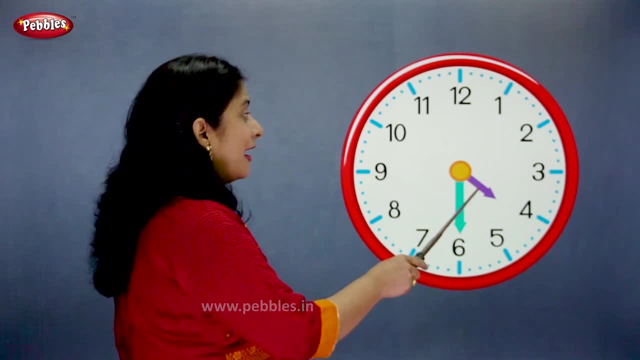 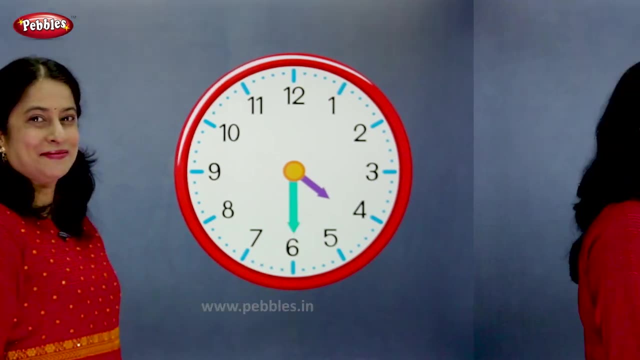 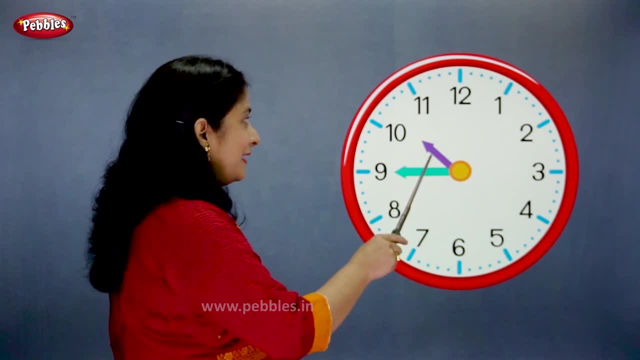 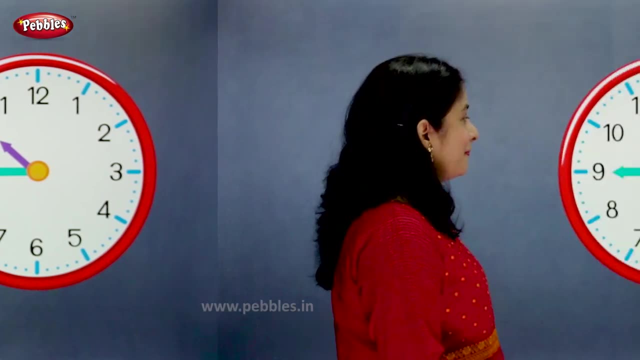 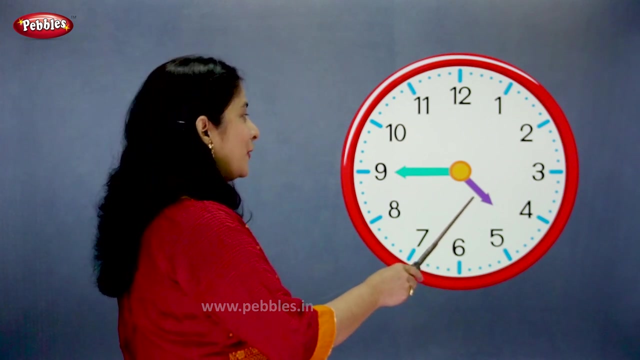 minute hand is on 9.. The hour hand is moving towards 11.. So we say the time is quarter to 11.. The minute hand is on 9.. The hour hand is moving towards 5.. So we say the time is quarter to 5.. 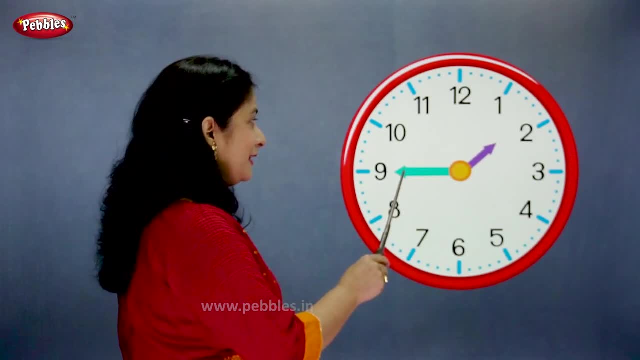 The minute hand is on 9.. The hour hand is moving towards 2.. So we say the time is quarter to 2.. The minute hand is on 9.. The hour hand is moving towards 7.. So we say the time is quarter to 7.. 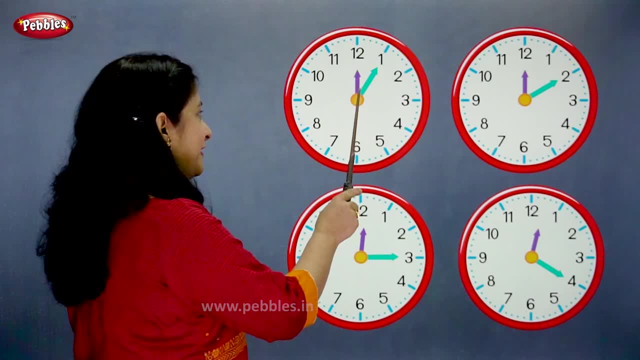 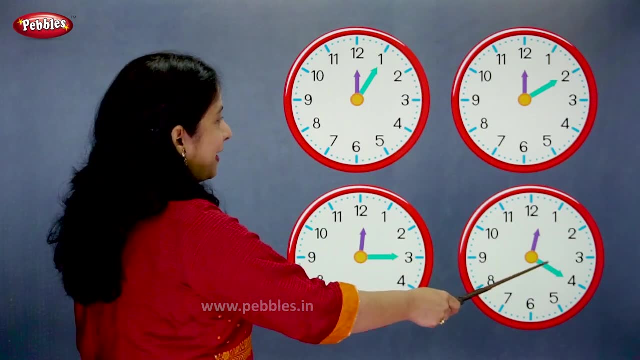 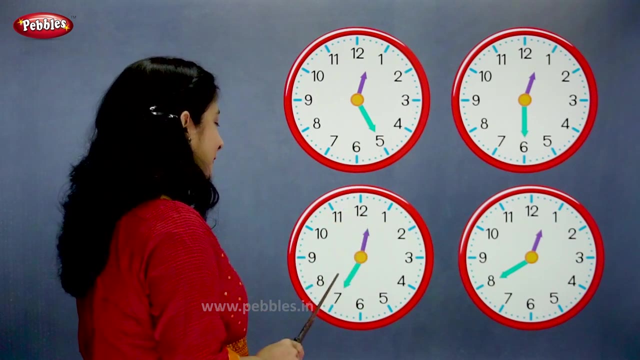 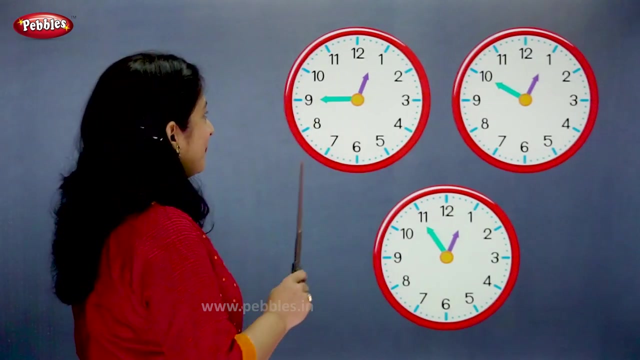 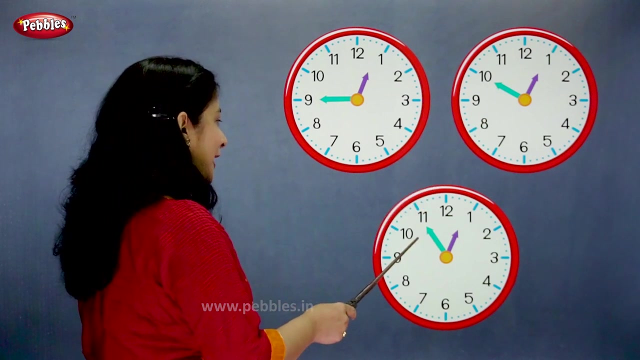 When the minute hand is on 1, we say 5 passed 10 passed Quarter passed 20 passed 25 passed Half passed 25, 2. 20, 2. Quarter 2. 10, 2. 5, 2.. 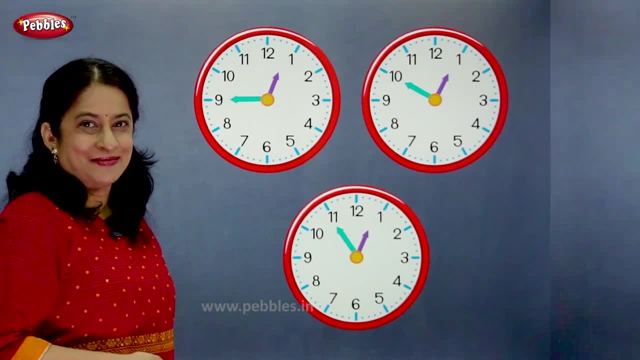 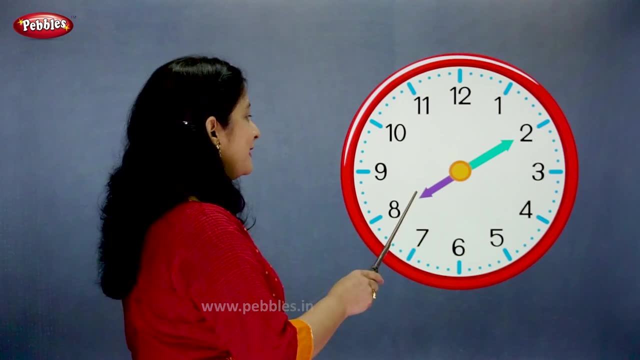 Now let's see some examples. The minute hand is on 2.. The hour hand is on 8.. So we say the time is 10 past 8.. The hour hand is moving towards 3.. The minute hand is on 10.. So we say the time is 10 to 3.. 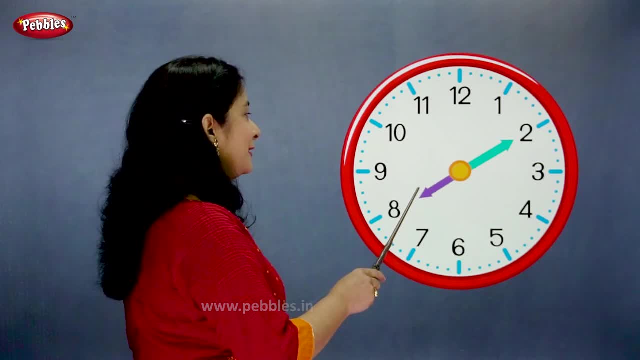 hand is on 8.. So we say the time is 10 past 8.. The hour hand is on 9.. The minute hand is on 8.. The hour hand is on 9.. The minute hand is on 8.. The hour: 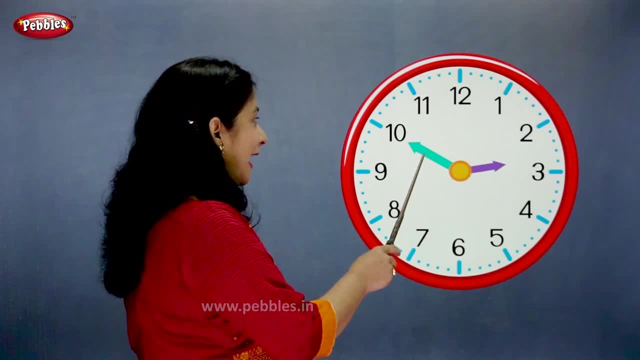 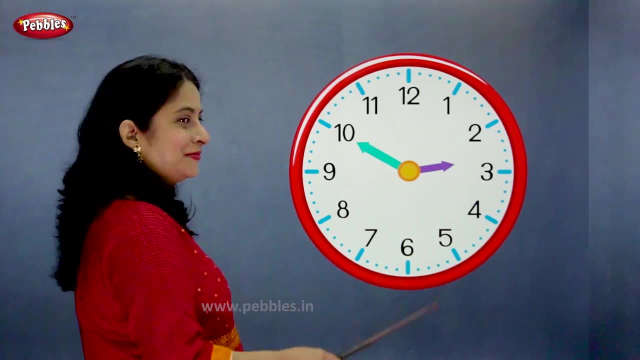 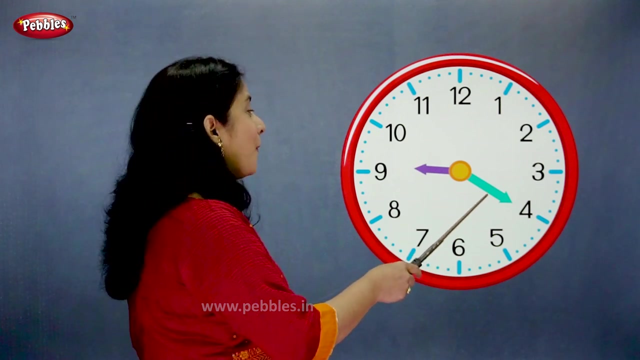 hand is moving towards 3.. The minute hand is on 10.. So we say the time is 10 to 3.. The hour hand is on 9.. The minute hand is on 4.. So we say the time is 20 past 9.. The hour hand is moving towards 7.. 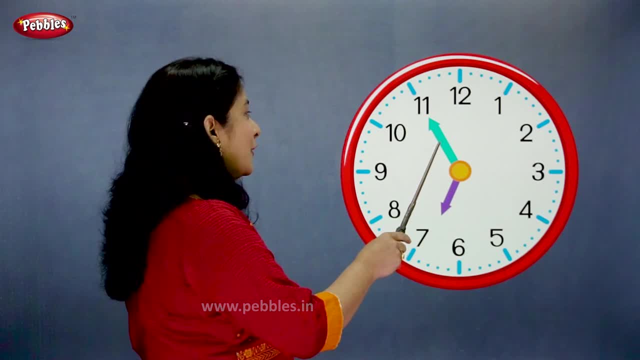 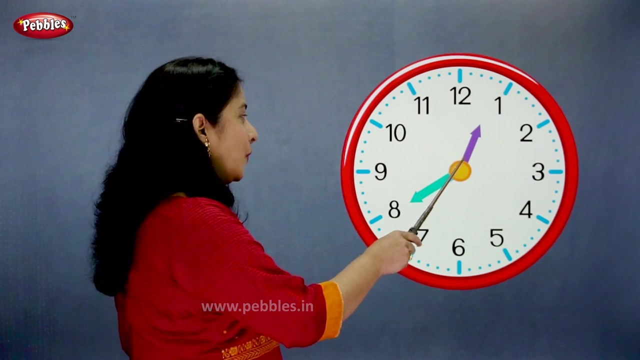 The minute hand is on 11.. So we say the time is 5 to 7.. The hour hand is on 10.. The minute hand is on 5.. So we say the time is 25 past 10.. The hour hand is moving towards 1.. 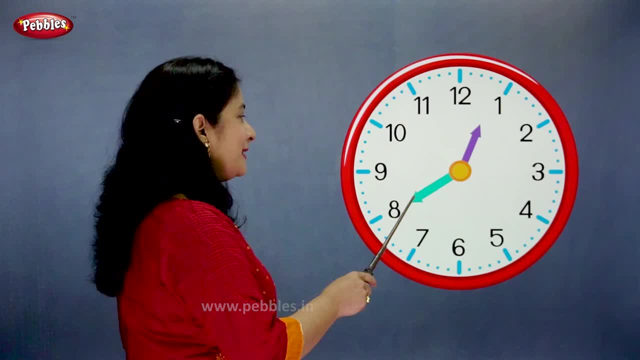 The minute hand is on 8.. So we say the time is 20 to 1.. The hour hand is on 6.. The minute hand is on 2.. So we say the time is 10 past 6.. Today we are going to play an interesting game. 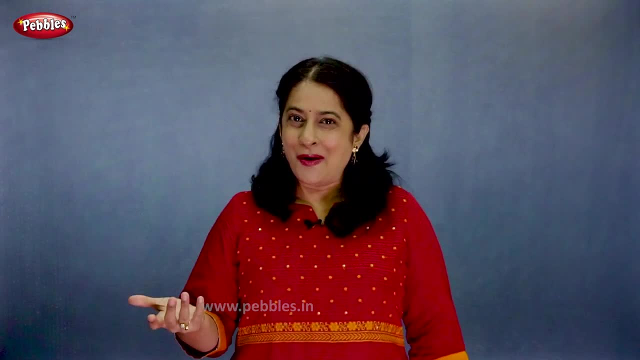 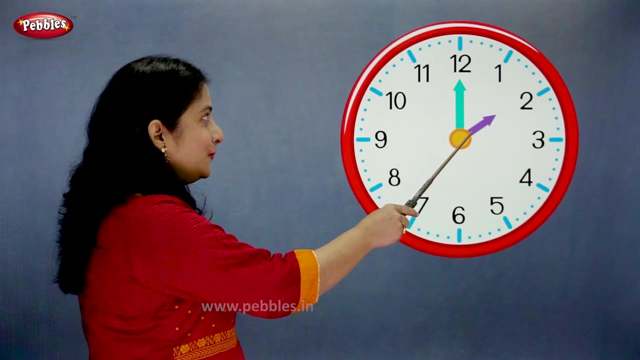 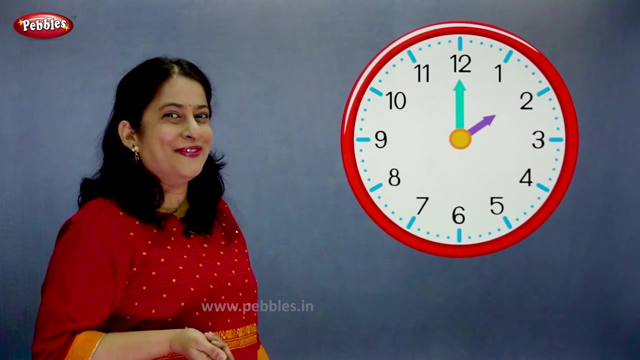 I am going to show you the various pictures of clock and you have to tell me the time. So let's start. The hour hand is on 2.. The minute hand is on 12.. So what is the time? Come on, tell me fast. 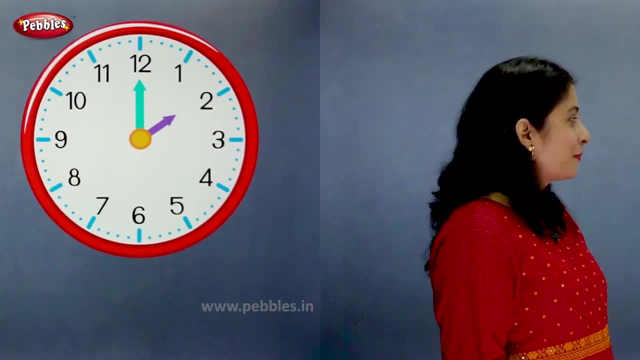 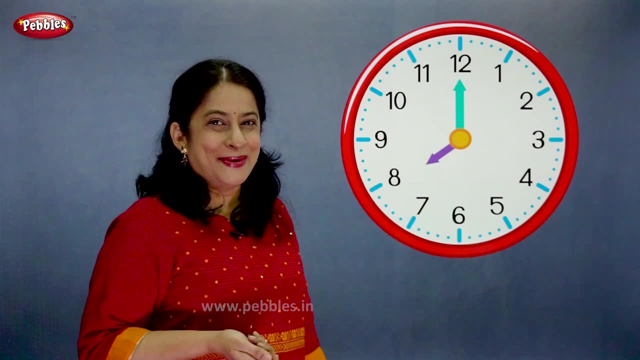 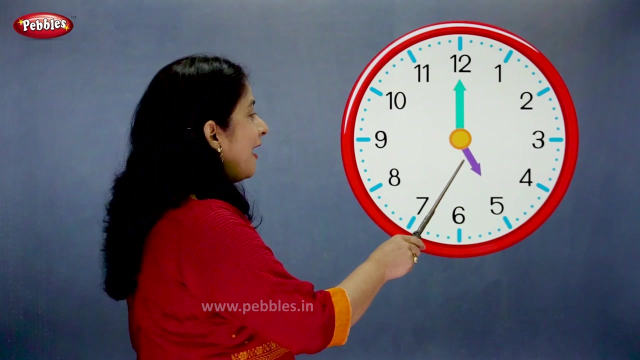 Correct: 2 o'clock. The hour hand is on 8.. The minute hand is on 12.. So what is the time Correct? The time is 8 o'clock. The hour hand is on 5.. The minute hand is on 12.. 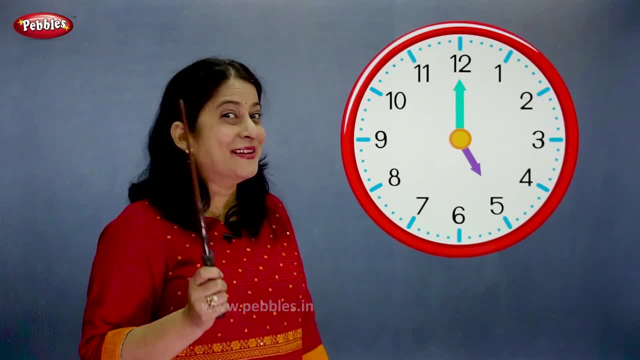 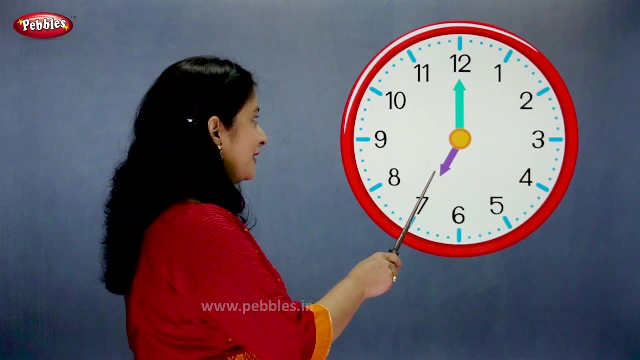 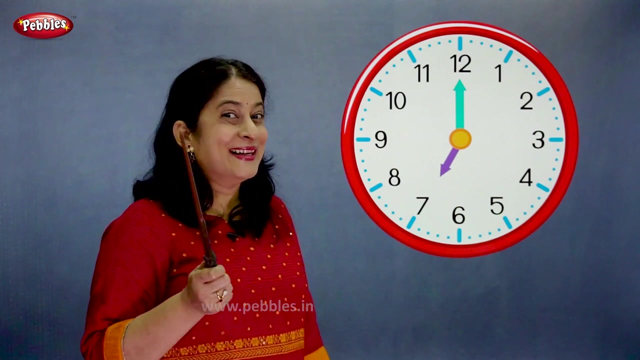 So what is the time? Come on, tell me. Right. The time is 5 o'clock, The hour hand is on 7.. The minute hand is on 12.. So what is the time? Come on, tell me fast. 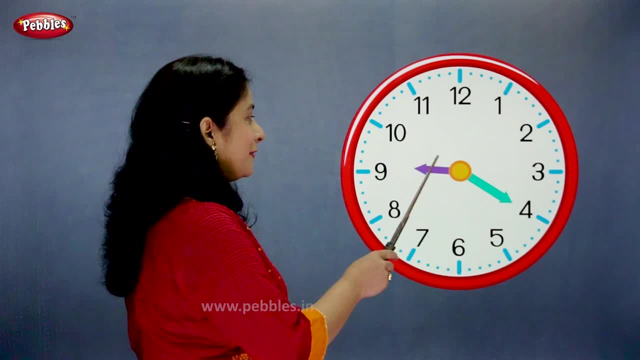 The hour hand is on 9.. The minute hand is on 10.. So we say the time is 10 to 3.. The hour hand is on 4.. So we say the time is 20 past 9.. The hour hand is moving towards 7.. The minute hand is on 11.. So we say the time is 5 to 7.. 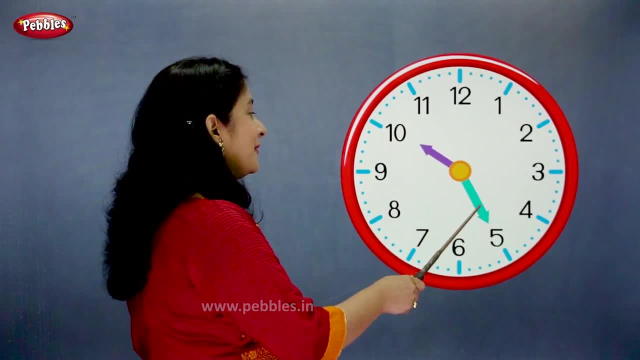 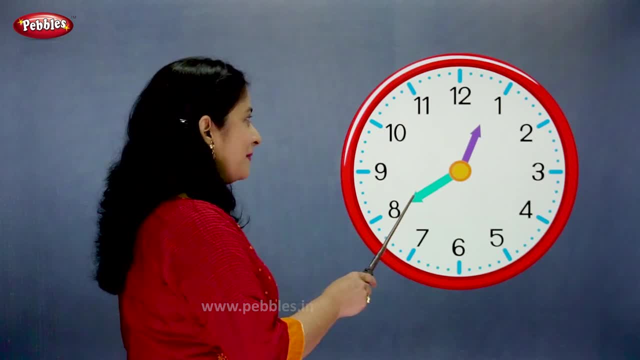 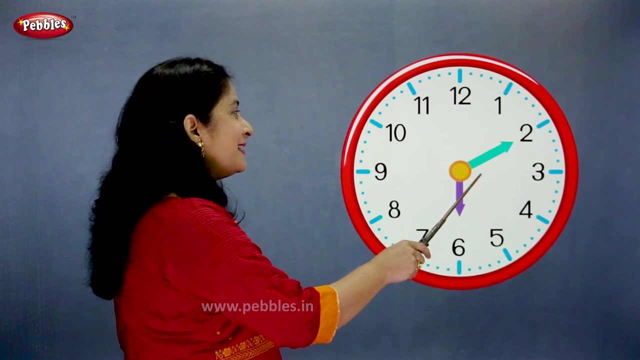 is on 8.. So we say the time is 20 to 1.. The hour hand is on 6.. The minute hand is on 2.. So we say the time is 10 past 6.. Today we are going to play an interesting game. I am going 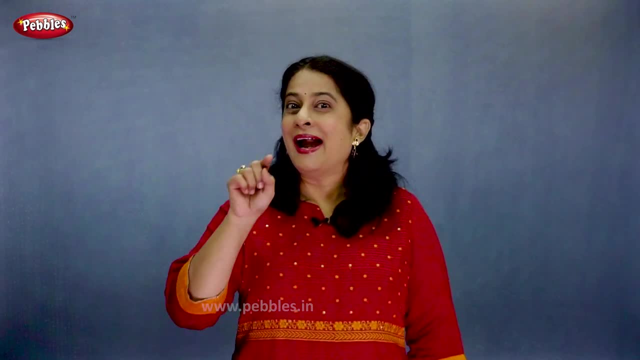 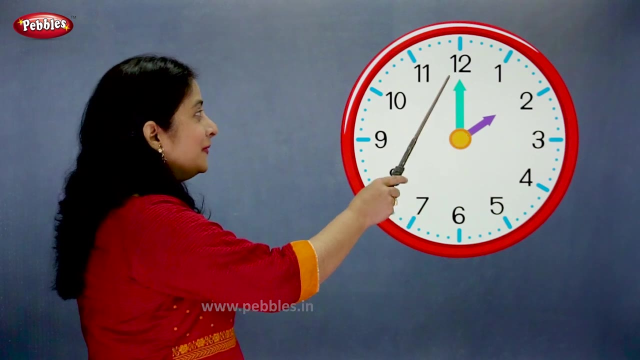 to show you the various pictures of clock, and you have to tell me the time. So let's start. The hour hand is on 2.. The minute hand is on 12.. So what is the time? Come on, tell me fast. 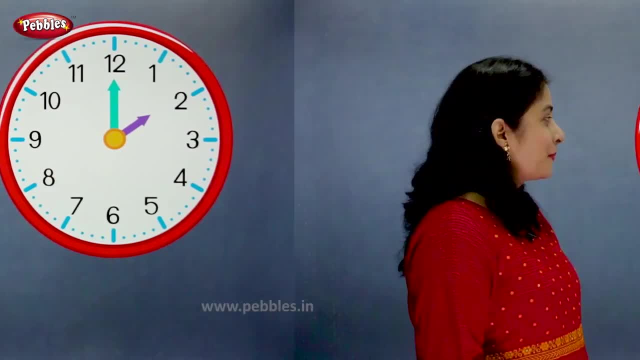 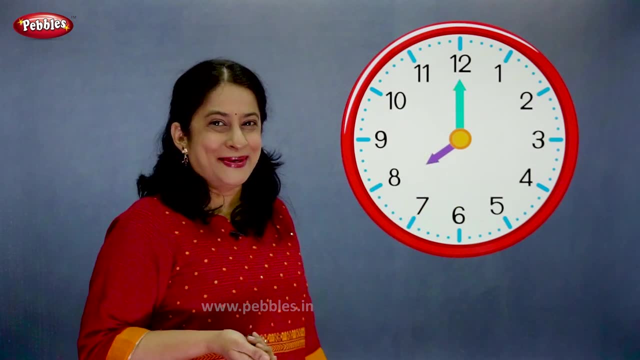 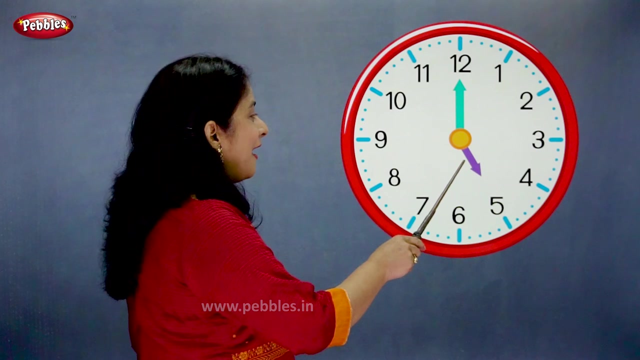 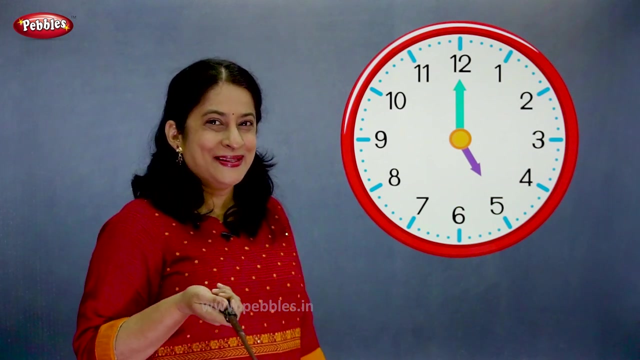 Correct: 2 o'clock. The hour hand is on 8.. The minute hand is on 12.. So what is the time? Correct? the time is 8 o'clock. The hour hand is on 5.. The minute hand is on 12.. So what is the time? Come on, tell me fast. 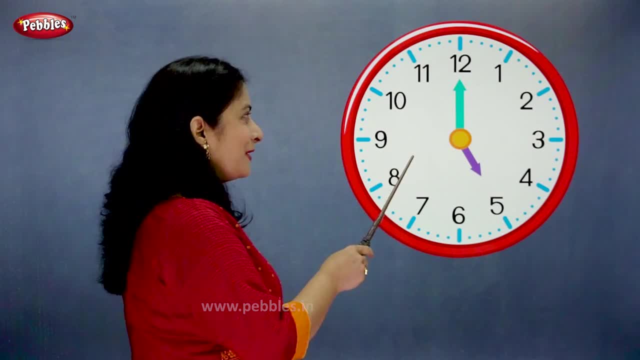 Correct, the time is 5 o'clock. The hour hand is on 7.. The minute hand is on 12.. So what is the time? Come on, tell me fast. Correct, the time is 7 o'clock. The hour hand is on 10.. The minute hand is on 12.. 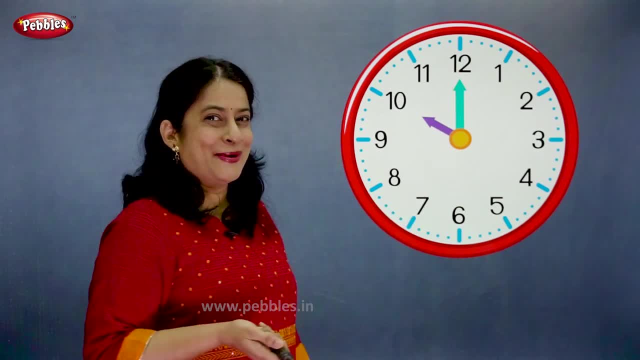 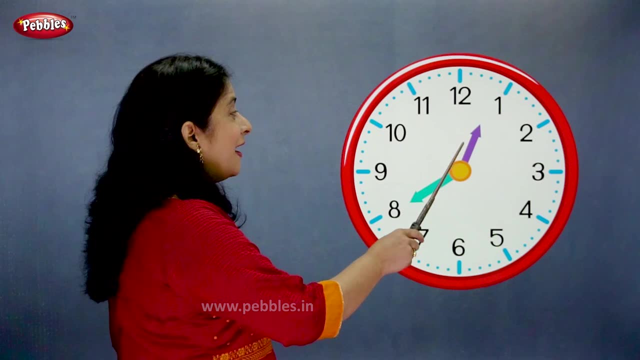 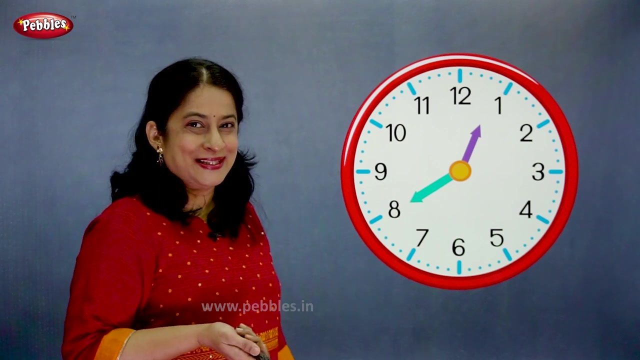 The minute hand is on 12.. So what is the time? Correct, The time is 10 o'clock. The hour hand is moving towards 1.. The minute hand is on 8.. So what is the time? Come on, tell me fast. 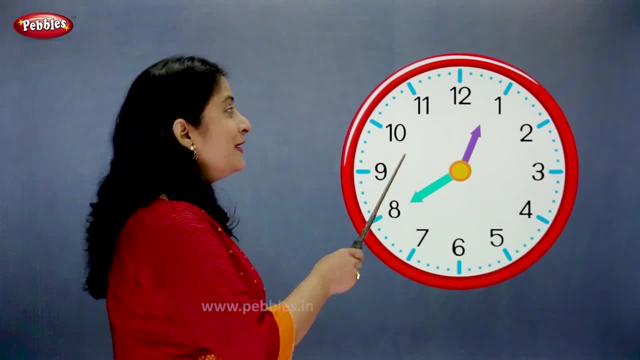 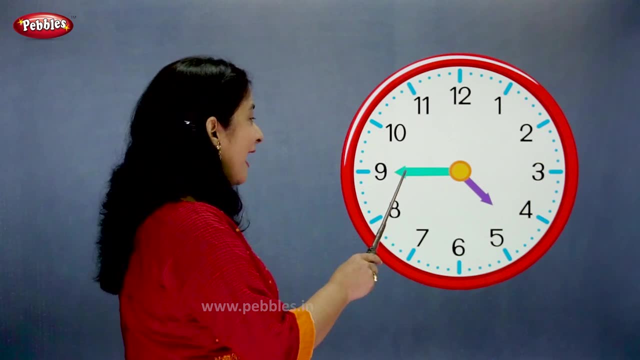 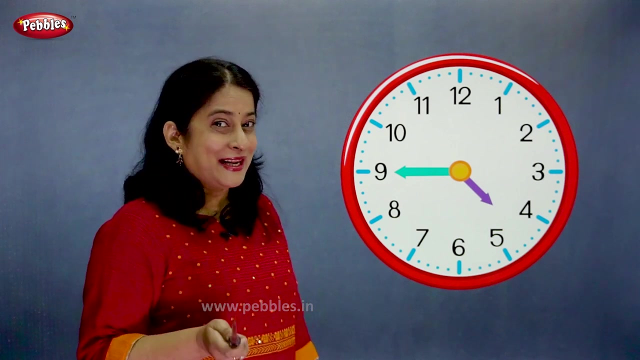 Correct, It's 20 to 1.. The hour hand is moving towards 5.. The minute hand is on 9.. So what is the time? Come on, tell me fast. Correct, The time is quarter to 5.. 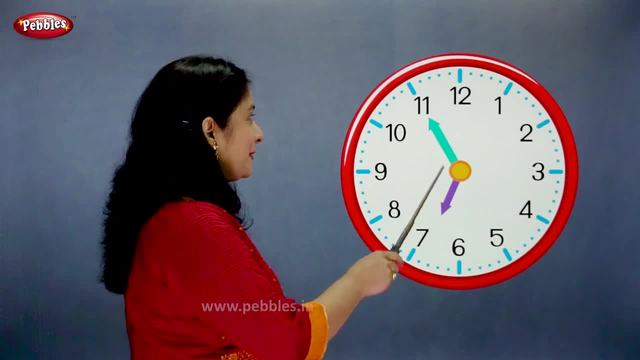 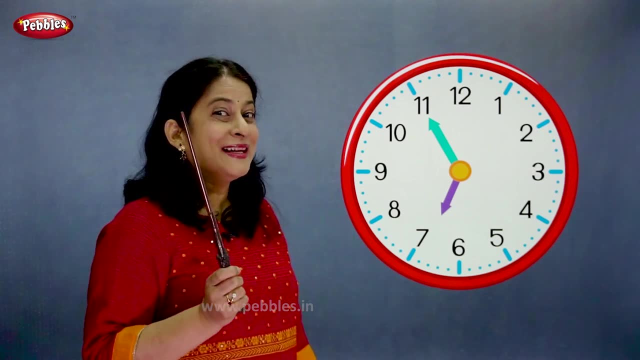 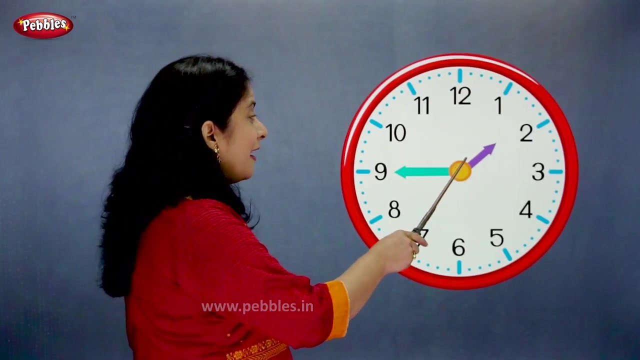 The hour hand is moving towards 7.. The minute hand is on 11.. So what is the time? Come on, tell me fast. Correct, The time is 5 to 7.. The hour hand is moving towards 2.. 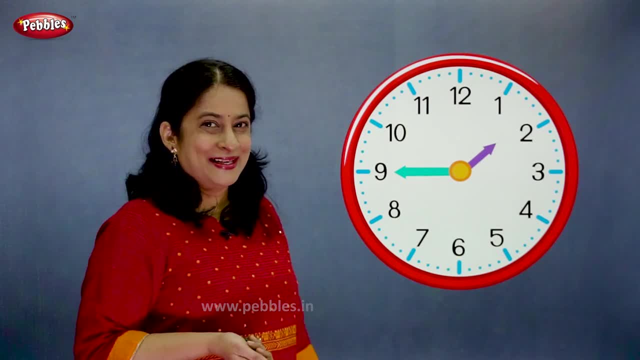 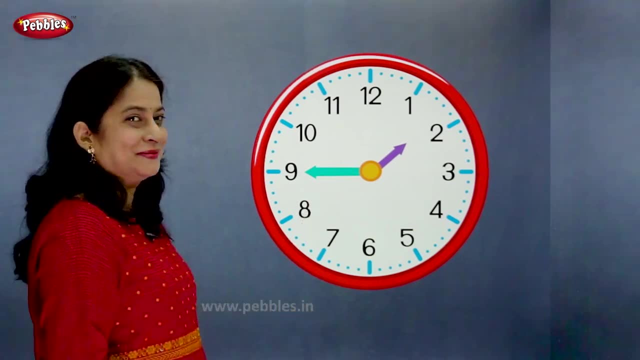 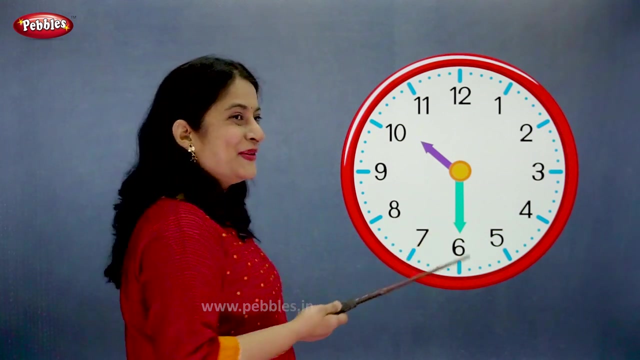 The minute hand is on 9.. So what is the time? Come on, tell me Correct. The time is quarter to 2.. The hour hand has passed 10.. The minute hand is on 6.. So what is the time? 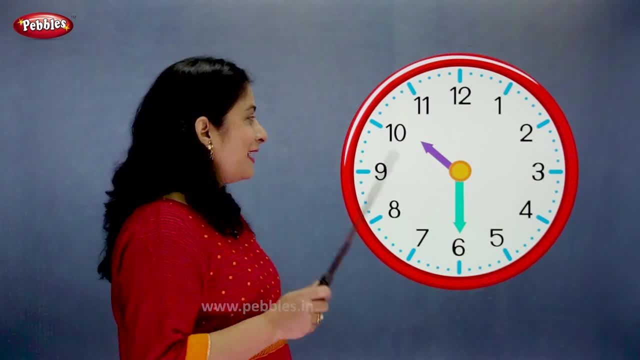 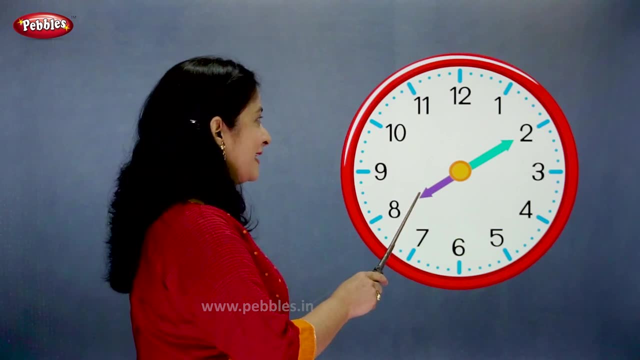 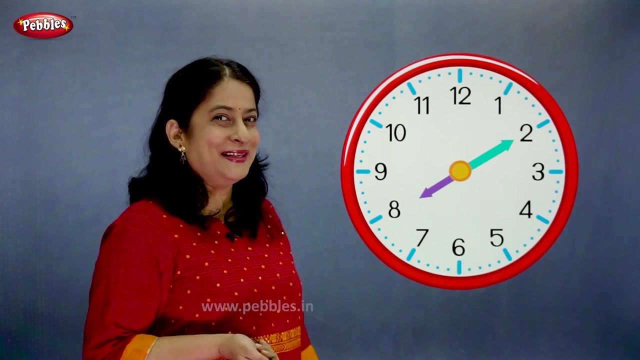 Come on, tell me fast, Correct. The time is half past 10.. The hour hand is on 8.. The minute hand is on 2.. So what is the time? Come on, who is going to tell me, Correct? 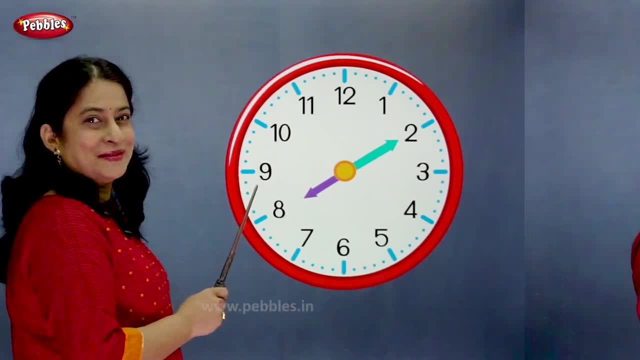 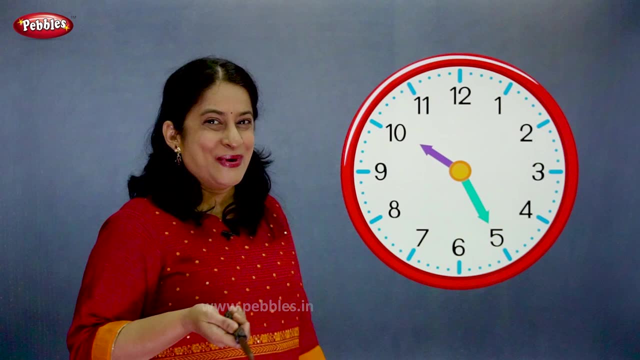 The time is 10 past 8.. The hour hand is on 10.. The minute hand is on 5.. So what is the time? Come on, tell me fast. Correct, The time is 25 past 10.. Thank you for watching the video. Please subscribe to our channel and press the bell icon. Bye.